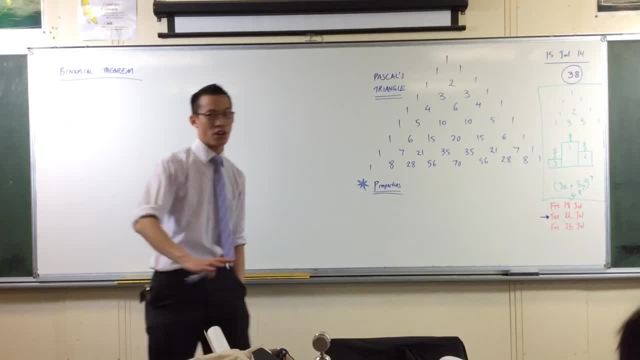 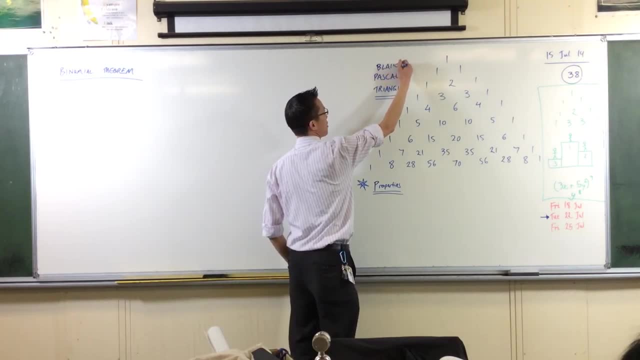 You can find it in all kinds of mathematical literature going back centuries. But Pascal did a lot of work with it And it's not just because he has a cool first name that it got named after him. It's largely owing to him. Like, come on, Who names their kid Blaise? 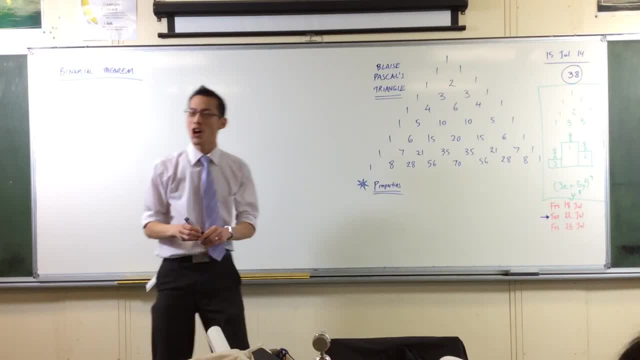 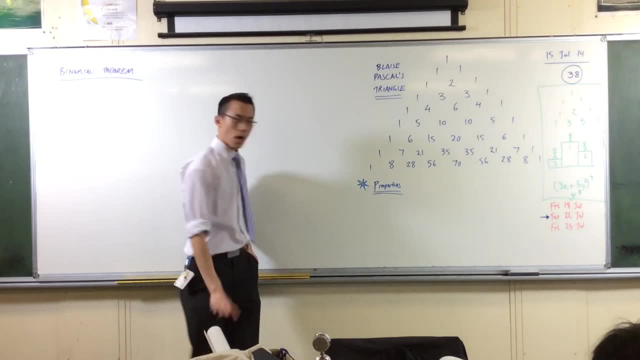 I'm going to call my kid Blaise, Those crazy French people, Anyway. So Blaise, Pascal and his triangle, Let's notice some things about it. Let's notice some things, For instance, What makes Pascal's triangle Pascal's triangle. 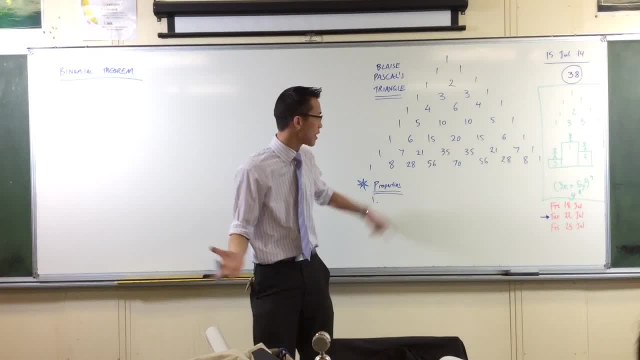 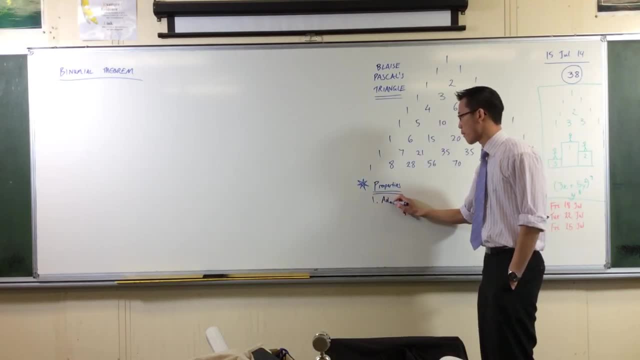 How is it constructed? This is the first property Like. actually, where do the numbers come from? They come from addition, right? In fact, the first and most important property is called the addition property. Right Now I'm not going to write it out and link it on the board because it would take me a while. 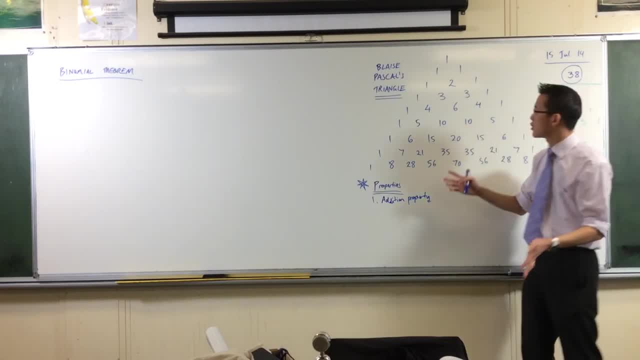 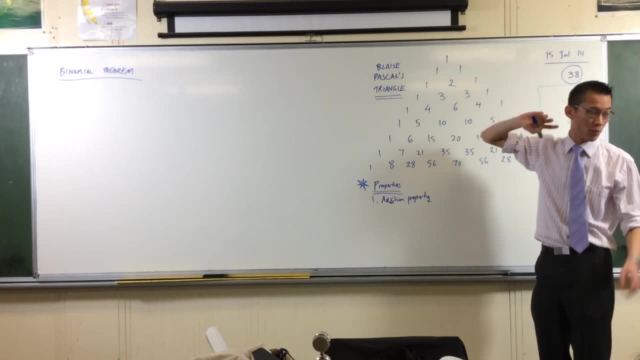 But I think you can see what it's getting at, right, With the exception of the first one right. And actually, if you put a different number up there as your starting point, your seed, if you like, you end up with a whole different thing. 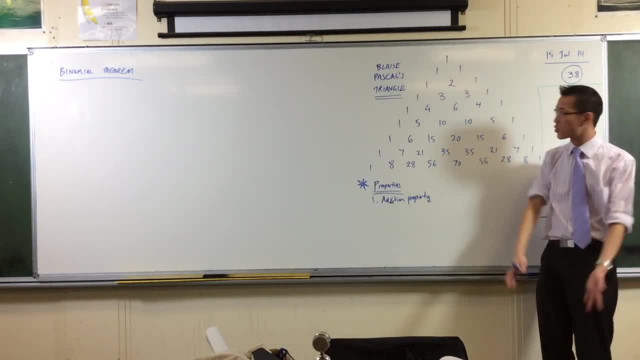 But anyway, Each number is composed of the two numbers immediately above it, Right, On its left and on its right, And in these cases there's no number on the left, So that's functionally at zero Right, Which is why it ends up as ones. 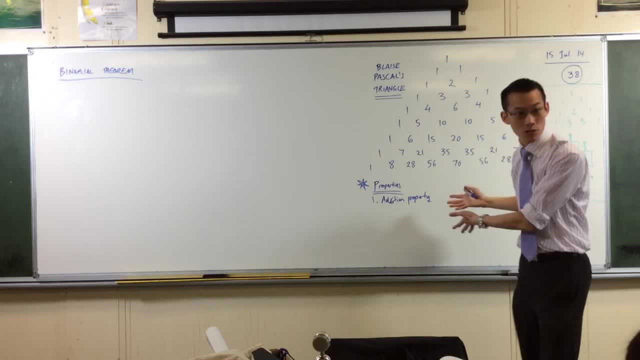 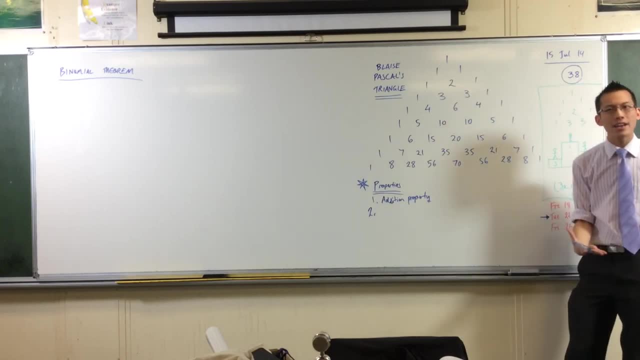 So the addition property is what makes Pascal's triangle Pascal's triangle. Okay, But there are other important things to note, Okay, For instance, If you have a look at the diagonals- And you guys have done this before, Right. 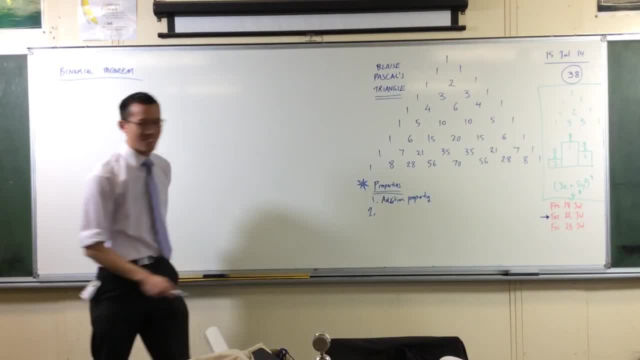 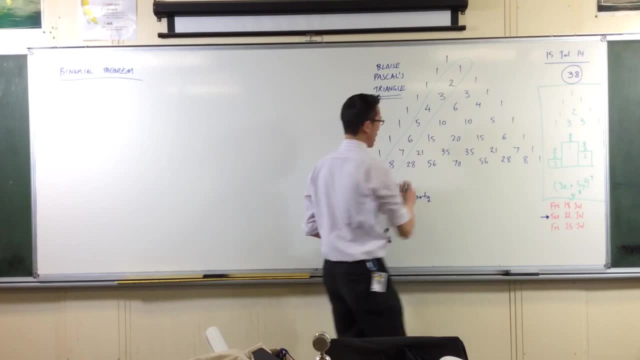 When you were just wee little people. The diagonals have properties, Okay, So I mean an obvious one If you take the second diagonal. Okay, What are those numbers? They're the counting numbers, Or the natural numbers, Or the set of positive integers. 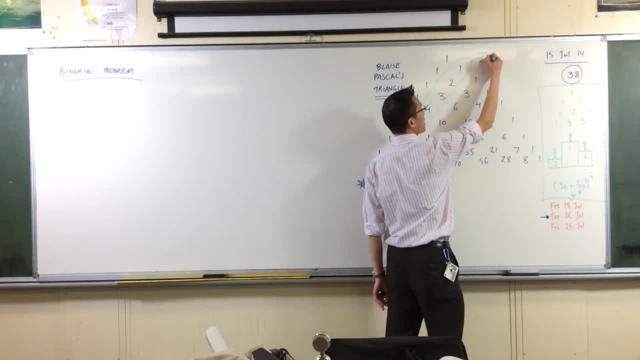 Right, So you have a pattern there, Right, But that's not the only pattern. For instance, If you take the next diagonal, This one is a little harder to recognise. Does anyone recognise what 1,, 3,, 6,, 10,, 15, and so on are? 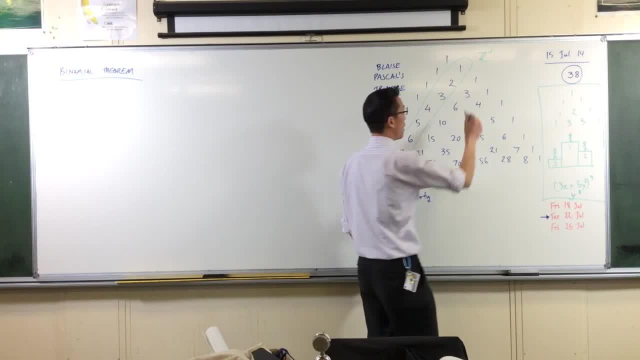 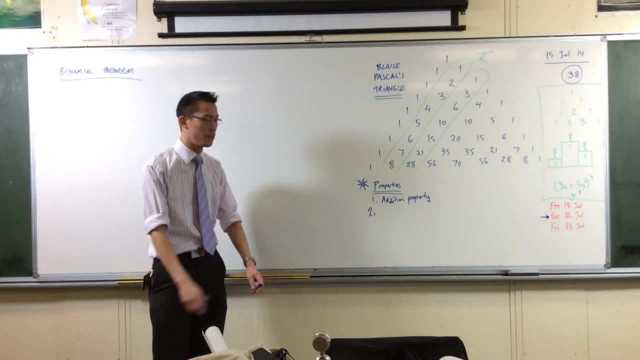 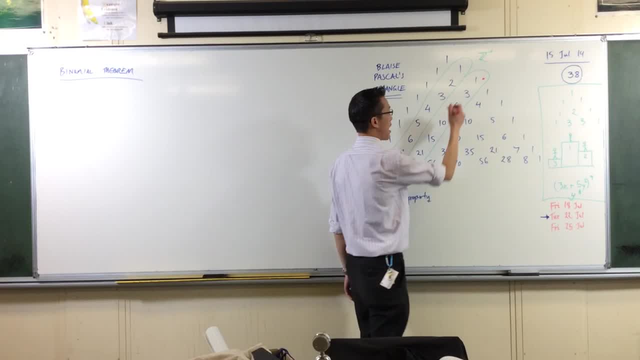 Yeah, Yeah, Right. Can you see the triangular numbers? Look, I'll show you. Here's 1.. Right Now, if I make a triangle, Here's 1,, 2,, 3.. Okay, And here is 1,, 2,, 3,, 4,, 5,, 6.. 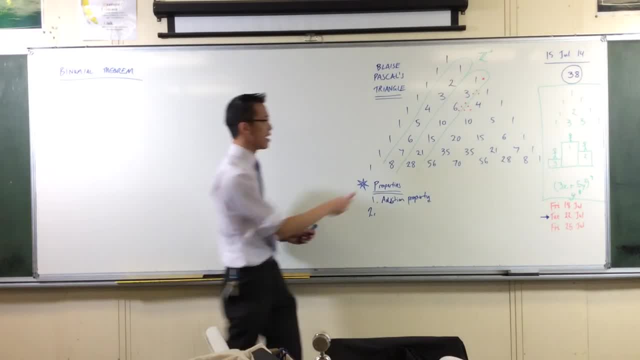 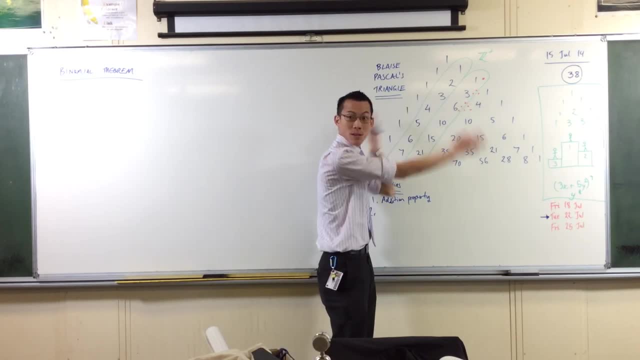 And I could keep going. Okay, Now, there's obvious reasons why this diagonal gives you the triangle numbers Right, Can you see it? It's because the triangle numbers are constructed in the same way that Pascal's Triangle is constructed. Okay, Not a coincidence. 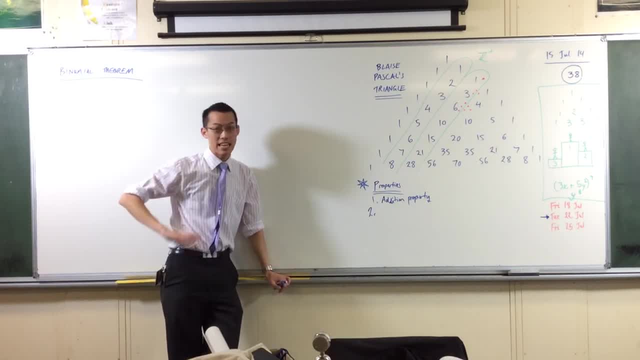 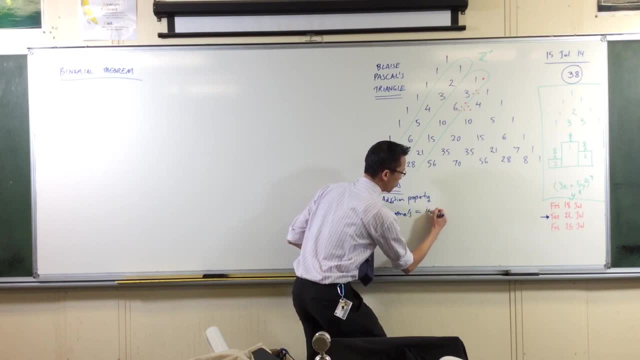 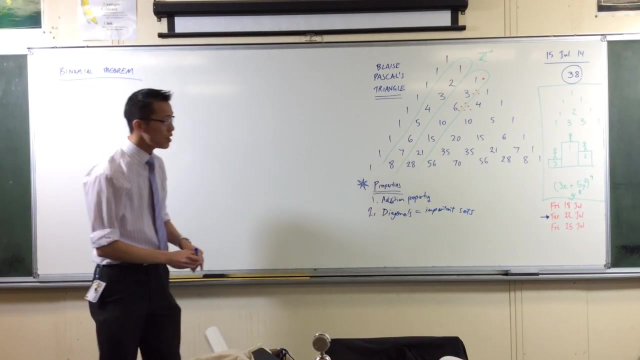 I wonder if you recognise what the fourth diagonal is. Okay, I'll let you have a think about it. So, number two, the diagonals. they are important sets, Those numbers, they're all connected, every single one. There's other interesting things about it. 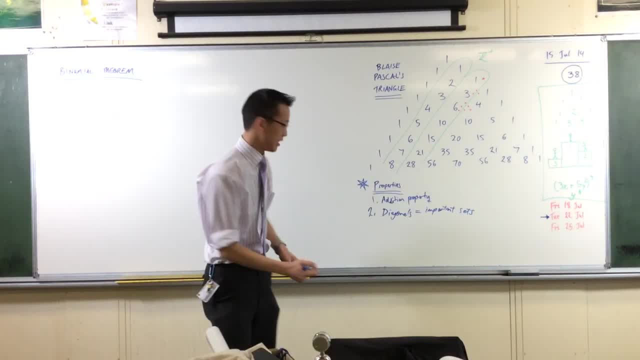 I've given you a couple. Can you give me some? What other kinds of properties can you see? I can see at least two more, Probably more, but what ones can you point out? I mean, some are obvious, right, When you add two numbers in the same row and you go down. 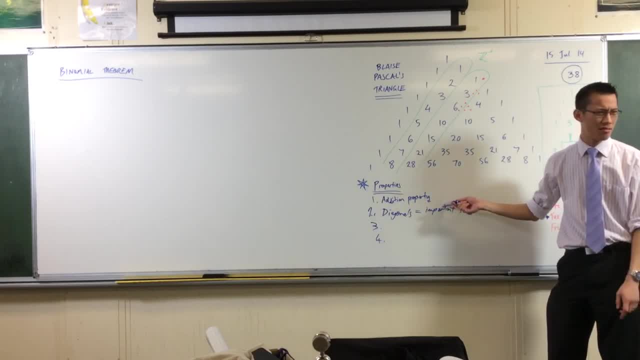 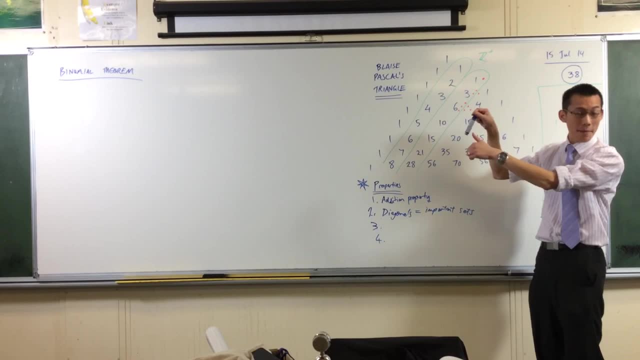 it's equal to that. Wait, that's this one, though, isn't it? Oh okay, Yeah, Hands up. if you missed me explaining what the first property was, Yeah, so the addition property it actually. by the way. 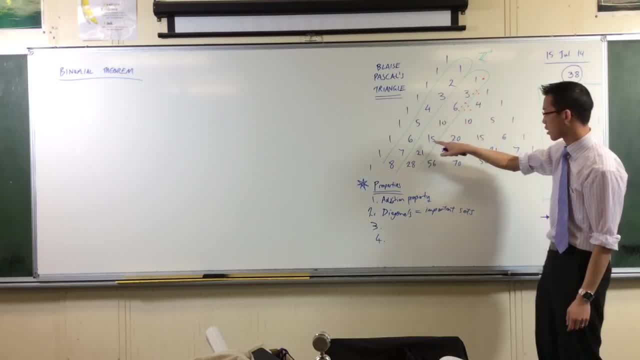 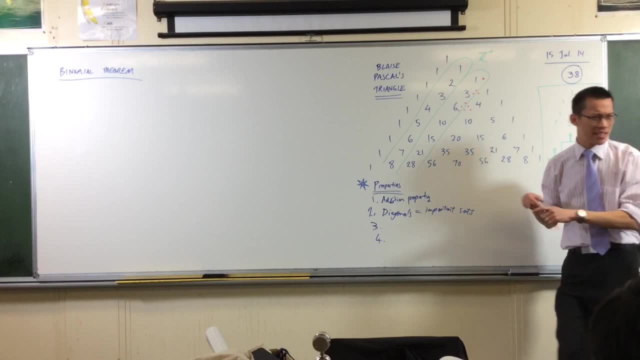 it feeds down further than just one row to the next. You can talk about two rows difference, and you can see that there are patterns there as well. obviously, And an obvious one: it's symmetrical. right, It's symmetrical. 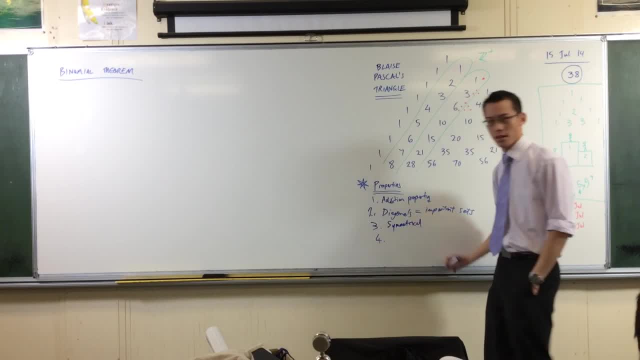 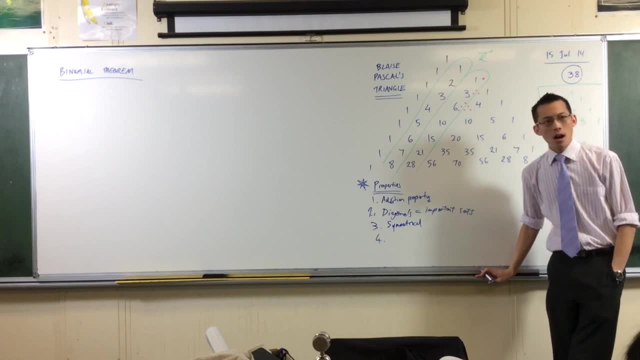 It has line symmetry. Each row is reversible. That's very important. You'll see why later on. okay, We've looked at the numbers and how they relate to each other, right. But if you have a look at the numbers and you add them up in different ways, 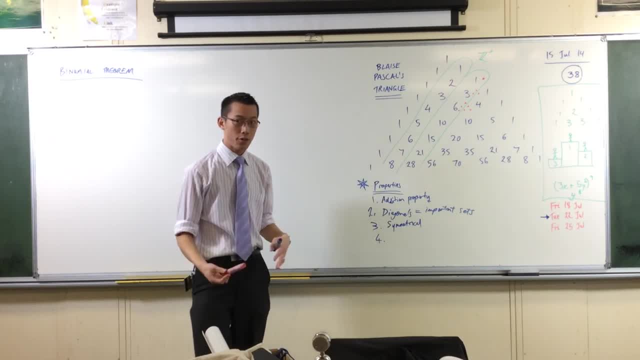 not just in the way that the addition property suggests: right, You get different things again. okay, For example: okay, the first row, the first row. What is the sum of all the numbers in the first row? It's one. 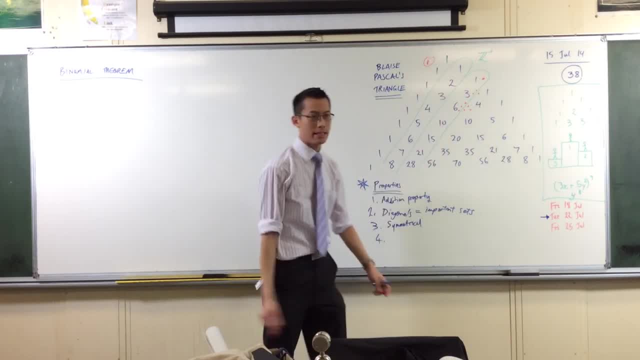 What is the sum of all the numbers? It's two. What is the sum of all the numbers in the second row? It's two, It's two. What is the sum of all the numbers in the next row? It's four.